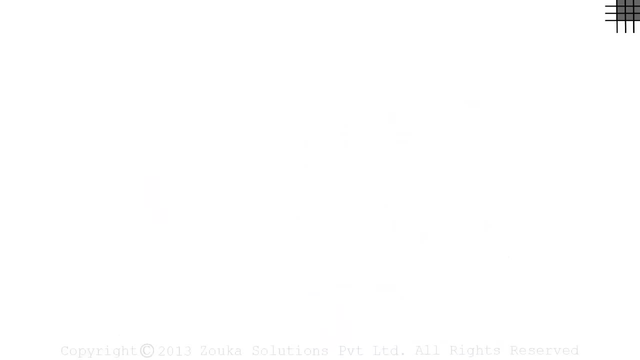 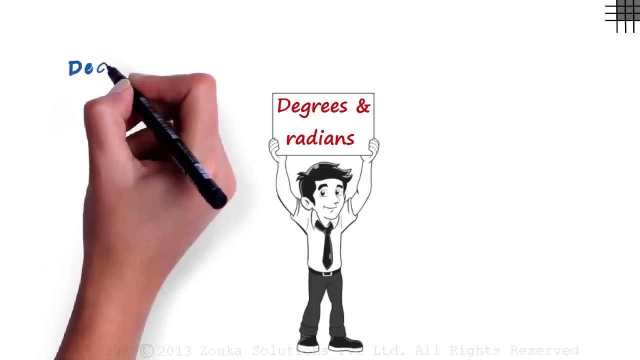 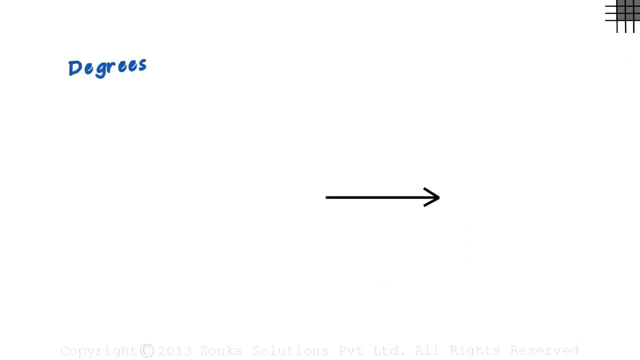 We know that angles can be measured in two ways: Degrees and radians. Let's understand degrees first. Angles are simply a union of two rays. Let this be one ray. There are two special kinds of angles which are used very often. One angle looks like this and it's called a right angle. 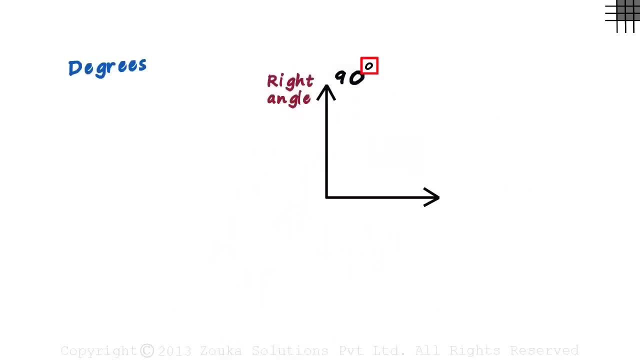 It measures 90 degrees. The small circle after the number is used to denote degrees, And do not confuse this degrees with the degrees we use to measure temperature. They are two different things. And the second special angle is the angle which forms a straight line. 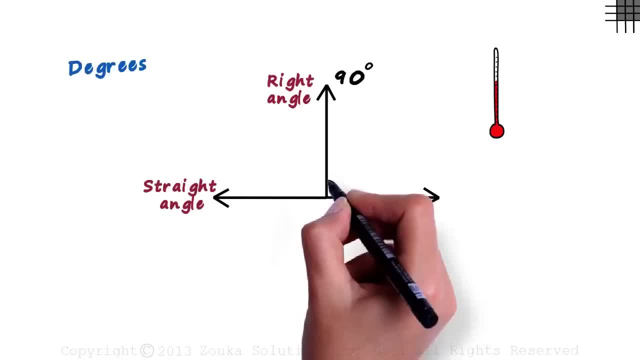 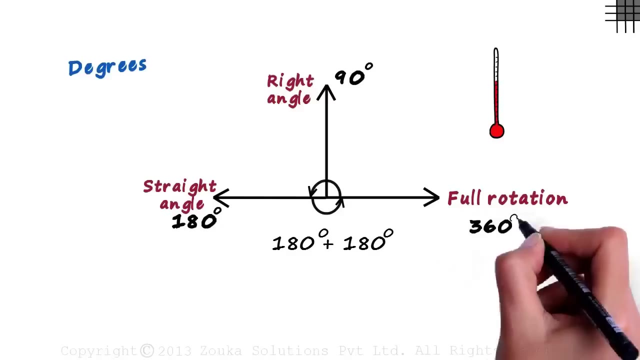 and is called a straight angle, And the measure of this angle is 180 degrees, And when this arm will rotate and overlap the initial arm, it is called one full rotation, Which equals 180 plus 180, 360 degrees. This brings us to the question. 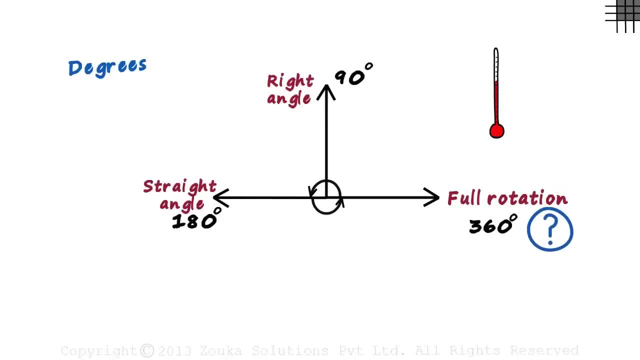 Why 360 degrees? Why not 1000 degrees? Because 1000 sounds very convenient to me. Why can't one full rotation be 1000 degrees? Well, think about it. I will probably be making another video to explain this. 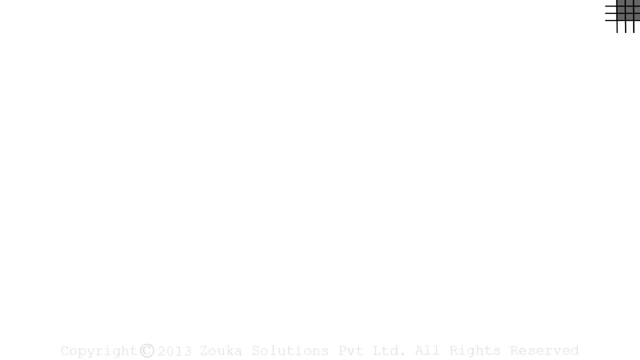 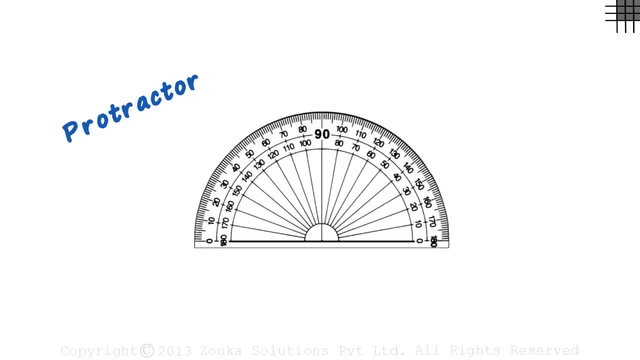 How do we measure or draw angles in our notebook? We use something called a protractor And it looks something like this: The numbers you see on the protractor are degrees. First let's see how we can measure angles using a protractor. 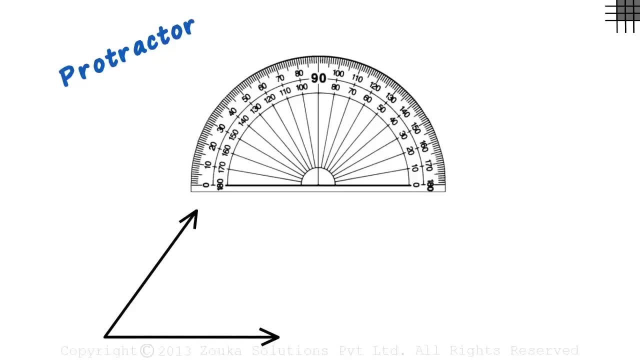 Let's say we want to measure this angle. To measure an angle, there are only two things we need to do. We need to keep this arm of the angle at the zero angle position and the vertex of the angle at the centre of the protractor. 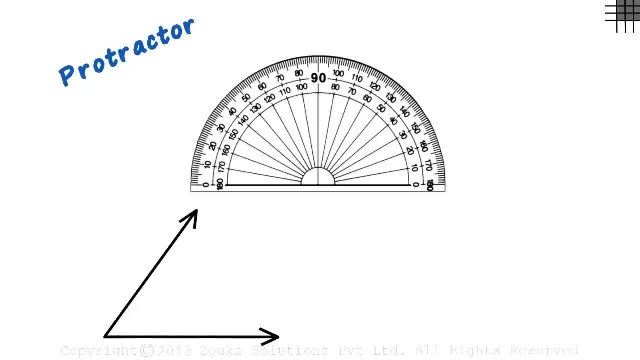 Normally we take the protractor to the angle, but in this video I will be taking the angle to the protractor Like this: Now we are in a position to measure the angle. This arm will be like our initial arm, which is the zero angle.